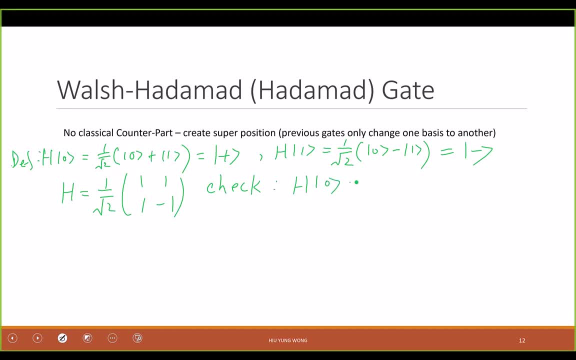 Example: Hadama gate. applied to 0 means it is 1 over square root 1, 1, 1, negative 1, applied to 0.. What is 0? again 1, 0.. When you measure 0,, what happens? 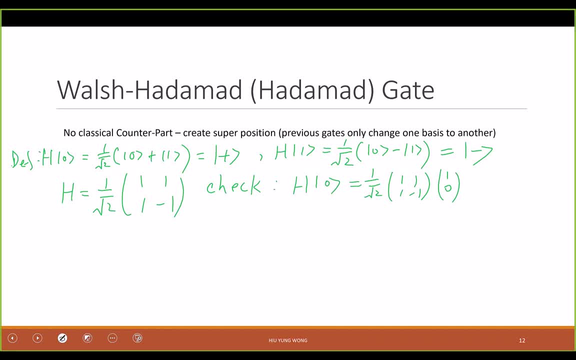 Not related to it. When you measure 0 states what happens: You get a 0. Okay, remember. okay, Exactly. I mean measure in the 0 and 1 basis. Good point, Okay, what is this? 1 times 1 plus 1 times 0.. 1 times 1 plus negative. 1 times 0, right. This is 1, 1, right, Which is equal to plus. Is that okay? 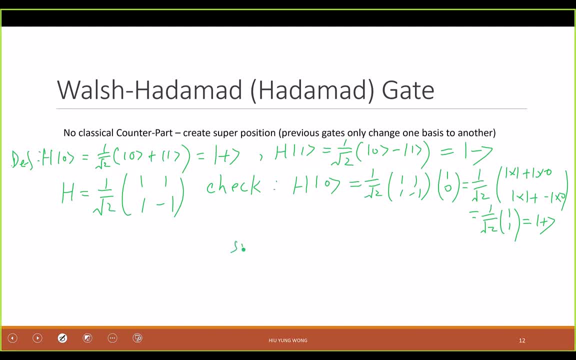 Right, so you can track yourself again. similarly, H applied to 1 equals to square root 1 negative 1,. right, You can check it. I won't show you here, but here I hope you can memorize. Memorize the definition. Why do you need to cheat sheet? Memorize it? It's easy for you compared to other classes. right, You know E124, you need to memorize the output impedance of common gates with degenerate, common source with degeneration. That's much more difficult, right, This is easy for you. 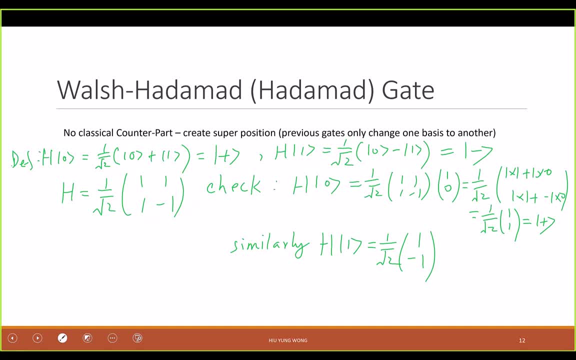 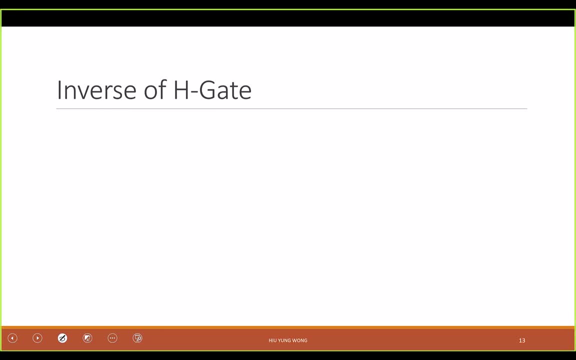 Easy: 1, 1, 1, negative, 1.. Memorize it, Okay here. I do want to say one thing about the inverse of the Hadamard gate, right? So inverse means what? The reverse direction? And it happens that inverse of the Hadamard gate equals to Hadamard gate itself. 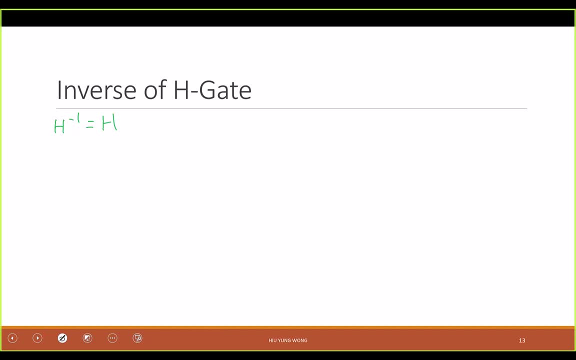 Okay. so if you have a circuit that starts with Hadamard gate and followed by inverse, it's just the same as two Hadamard gates. Okay, so let me prove to you that it is true. First of all, we also take this opportunity. 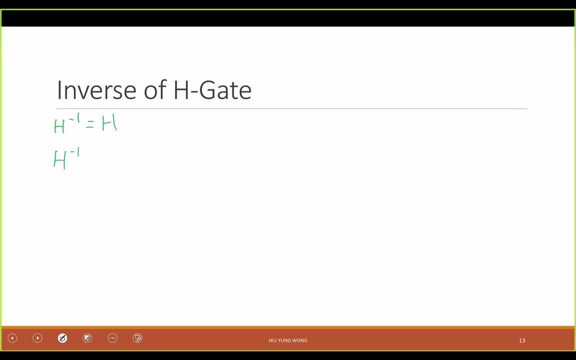 to review how to find the inverse of a matrix. The inverse of matrix is 1 over the determinants of the matrix. This absolute value means determinants. It's okay, you forgot what is determinants. You can always Google And then inside the 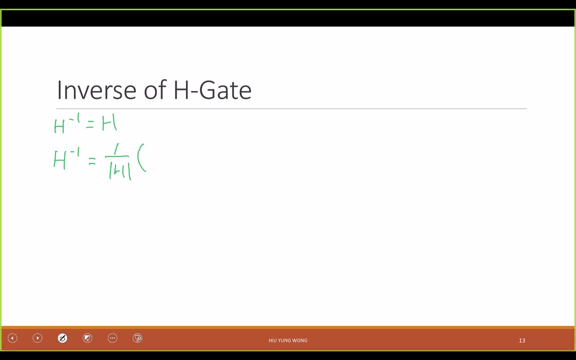 matrix. you have this so-called cofactor and minor negative, 1 i plus j, and then the m i j transpose. right, Let's write it down first, and then I will define this to you. I make it so complicated because this is the general expression for the inverse It might be. 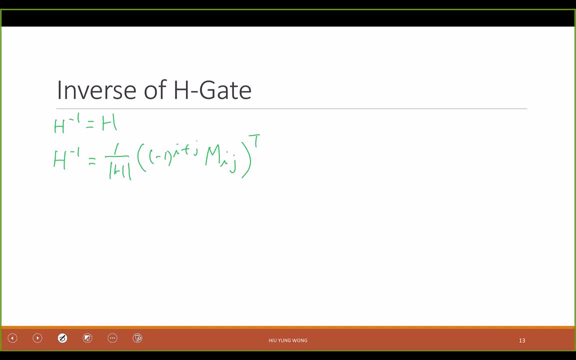 useful when you do two qubits or more. We won't use that much, but I want you to be aware of this complexity of the inverse For a 2 by 2 matrix. it is easy, right? So what is that? First of all, 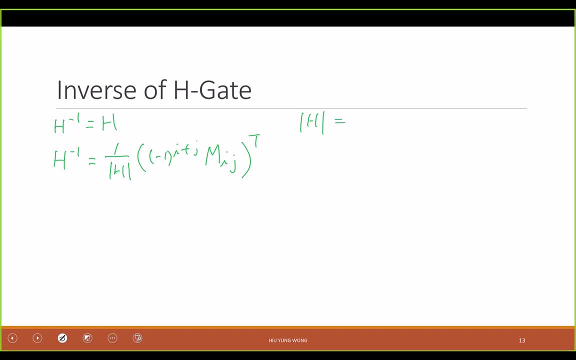 let's find the determinants. The determinants is also complicated, right, But for 2 by 2, it's easy. The determinants is what? Let me just remind you, the Hardhamer gate is 1 over square root: 2, 1, 1, 1, negative: 1, okay, So the determinant is 1 over the square. 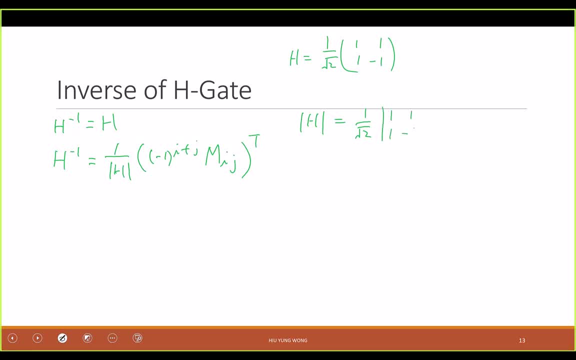 root 2, and how do you do it? Remember Very good, right, It is 1 times negative, 1 minus 2.. minus 1 times 1, right, You go in this diagonal minus the diagonal in other direction, and this: 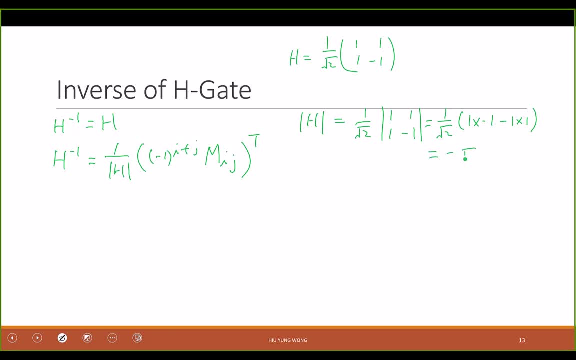 is equal to negative square root 2,, I believe. right, Because this is negative 2.. Is that okay? I will slow down a little bit. Is that okay? What do you think? Yeah, minus 2 over root 2 is what 2 divided by root 2.. Negative root. 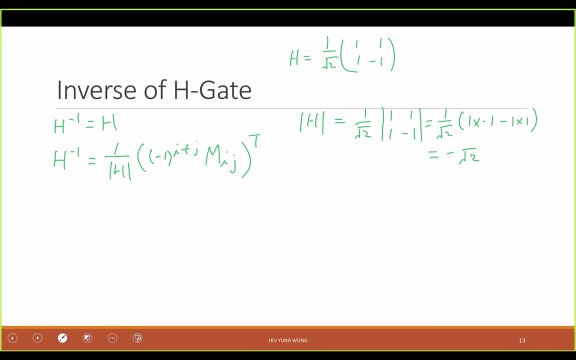 2, right, Okay, Good, Okay. so then, what is the meaning of this guy? This is talking about the I and J elements. right, I row J, column. Okay, First look at M00.. How do you find it? 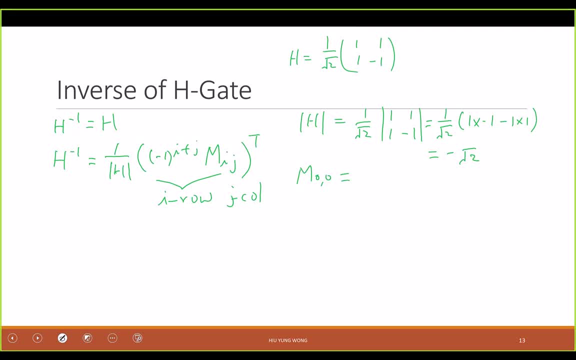 The way you find it is: just draw a line. Maybe let me show you You do this. 00 is where This is, 00, right. So remove this line, This guy, remove this column, Okay, And then you find out the determinants of the rest. 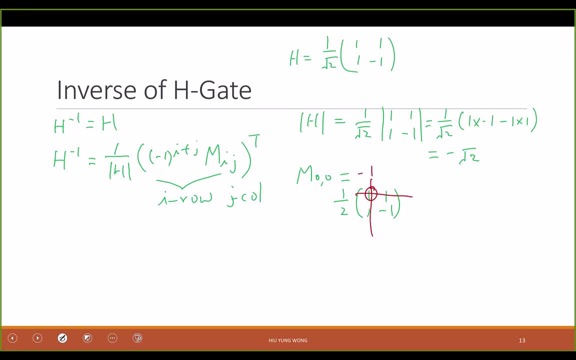 Okay, so this is negative. 1. How about M01?? Let's look at it again. What, which one is our target? 01. 01. This one right. Remove this row. This one, This one, This one. 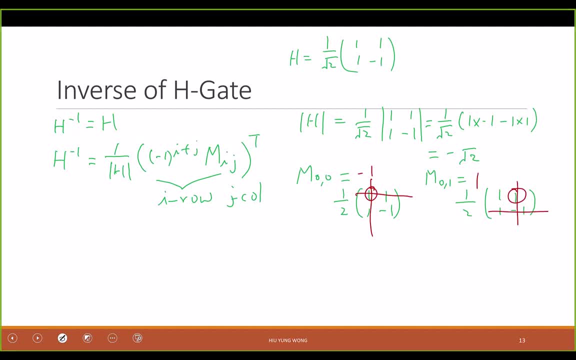 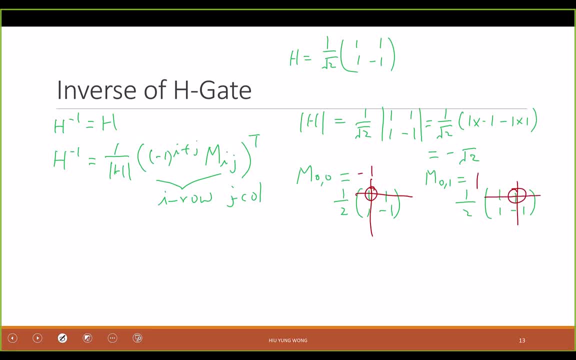 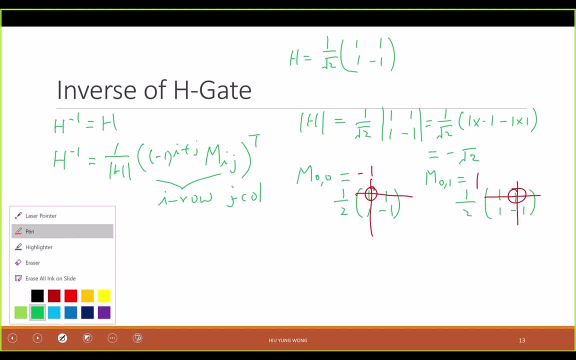 negative one left: M10. 10.. What do you get? 10. This is 10.. Right, So you get 1.. The 1 is left, okay, And eventually M15.. M11 equals to what is M11?? 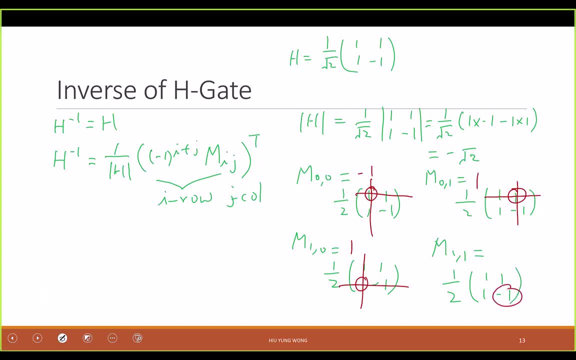 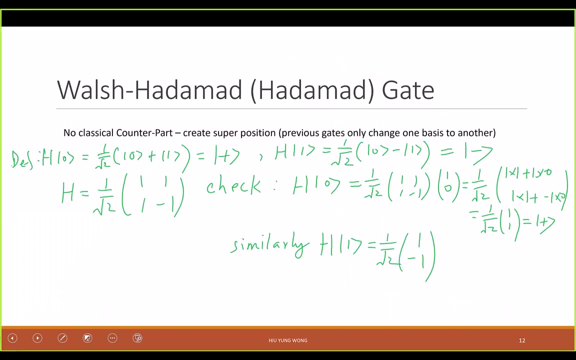 That is the mistake I made just now. right, It's: 1. Okay, Say again, Oh, yeah Again. that is typo, not half. That should be square root. 2. Yeah, and then I think I missed a lot of stuff. Hold on. 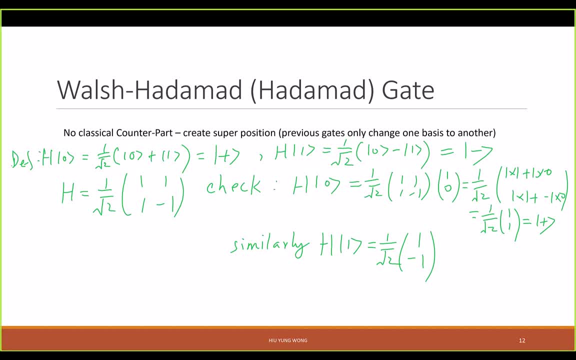 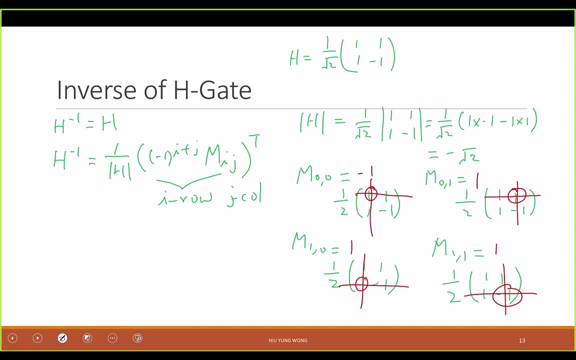 Sorry. So I missed a lot of stuff, actually Sorry for that. So should not be 1, right. Should be 1 over square root 2.. 1 over square root 2.. Is this okay? Because this is the whole matrix, right, The whole matrix: 1 over square root 2.. 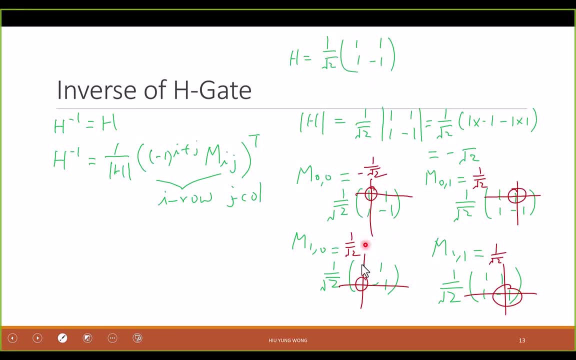 Right, You can just put 1 over square root 2 inside Instead of 1.. I missed the 1 over square root 2.. The whole thing is wrong. Okay, Yeah, if I did not have this 1 over square root 2,, I was right. 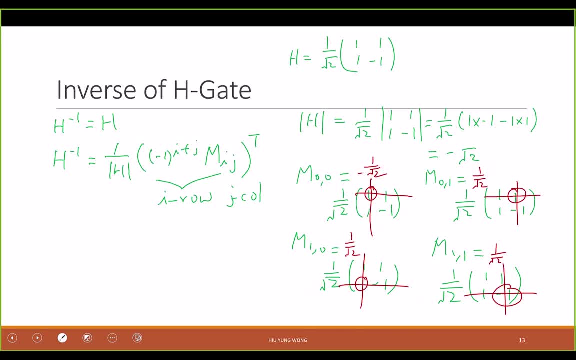 Negative: 1, 1, 1, right, But now I have 1 over square root 2.. So I need to multiply by 1 over square root 2.. I made the mistake. First of all, it's 1 over square root 2, not 1 over 2.. 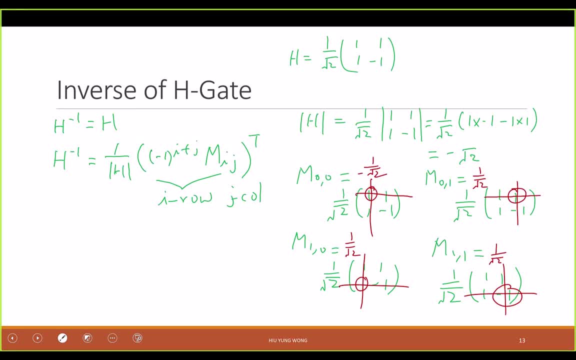 So you're definitely: before what, Before what? The whole thing, Yeah, the whole thing, Yeah, The whole thing. No, I'm only talking about m i j Yeah, m i j Okay. That's how you find the. 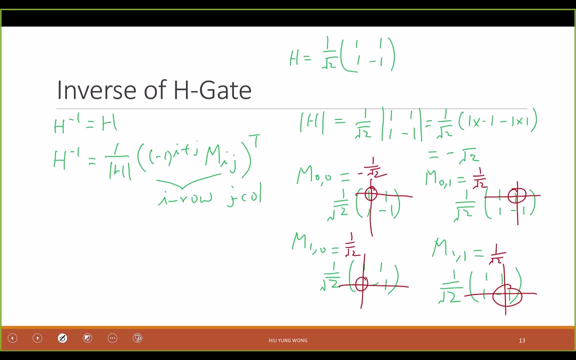 minor. Okay, Okay. so then what is the result? 1 over. This one is 1 over. I hope I'm right 1 over, because now it's completely different from my cheat sheet. Negative square root 2.. Good, thank you. 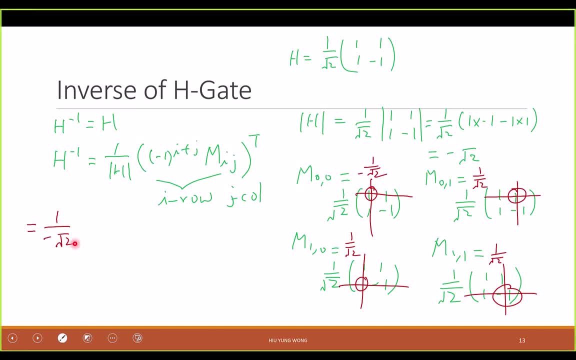 This is okay: 1 over h Right, 1 over negative square root 2.. You need to be very careful. I also saved the transpose. I don't do it yet. The first one is 0 plus 0.. So this negative to the power. 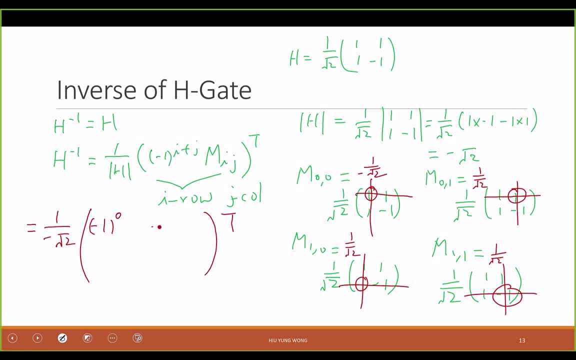 0. Right. The second one is negative: 1 to the power: 1. Negative 1 to the power: 1. Negative 1 to the power: 2. Right For this cofactor. Okay, And then what is m i j? 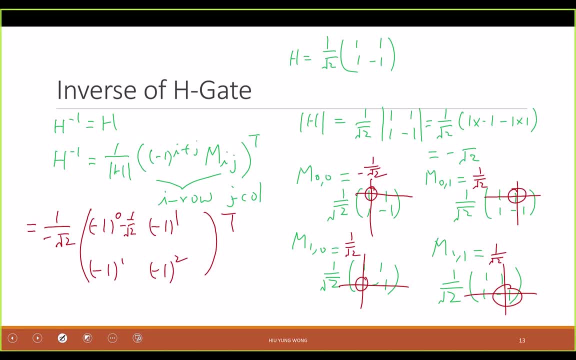 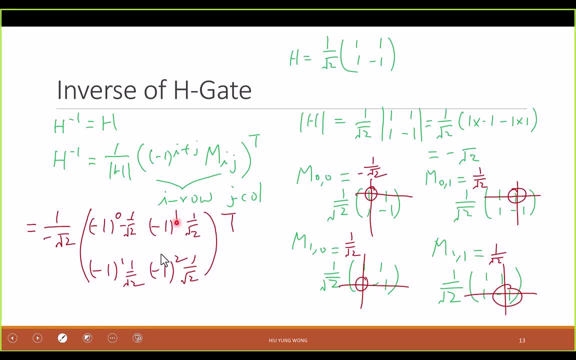 the transpose because obviously they are symmetric, So this transpose can be gone when I swap them. So I'm going to take out negative 1 over square root 2.. Okay- And I think I really make a mistake here- The Harder-Merger. Let's. 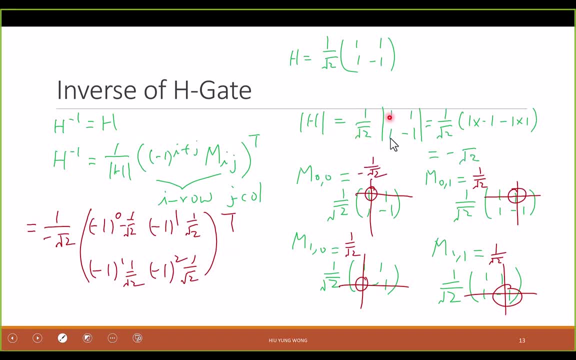 check Right. The Harder-Merger determines, if this times negative, 1 minus 1. So it's negative 2.. So negative square root 2.. So I put negative square root 2 here. Yeah, 1 over square root 2.. 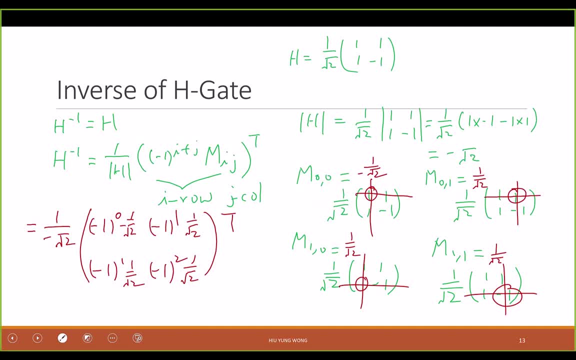 Yeah, but I think that I couldn't understand. Yeah, but the matrix you just think about should put the 1 over square root 2 inside, Right? Just factor it out. The whole matrix is 1 over square root 2.. 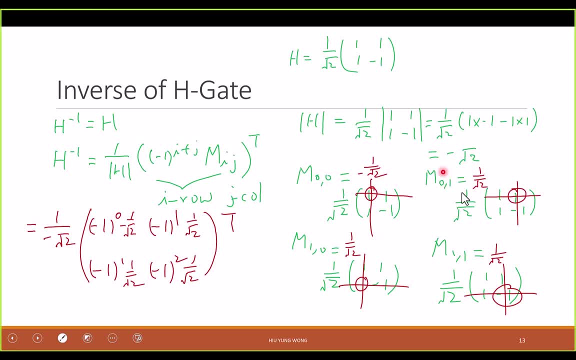 Yeah, in my cheat sheet I did put this as negative 1.. But that it looks like. What did I do wrong? No, transpose, it just switched. I still have 1 over square root 2.. Supposed to look like this one. 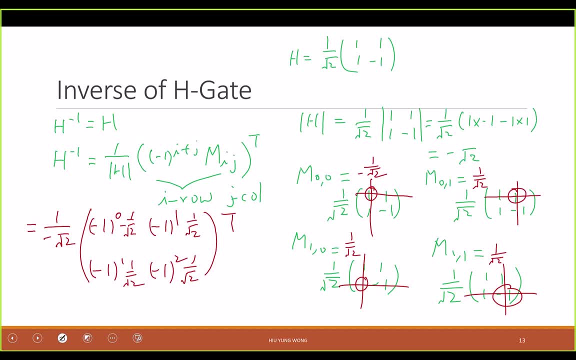 Yeah, Yeah, if I take this 1 over square root 2, negative 1 out Right, Then this become 2.. Right, This negative 1 over square root 2, they all take out Right And I take negative. 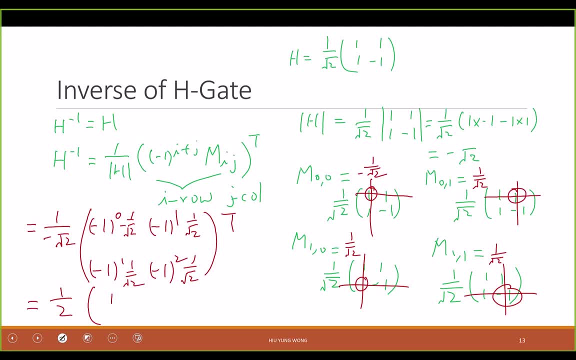 out. So this is 1.. This is also 1.. Because this is negative. This 1 is negative. Right, Then it should be equal to h, But So I think it's. That's right, But is it? I do something wrong about the determinant. 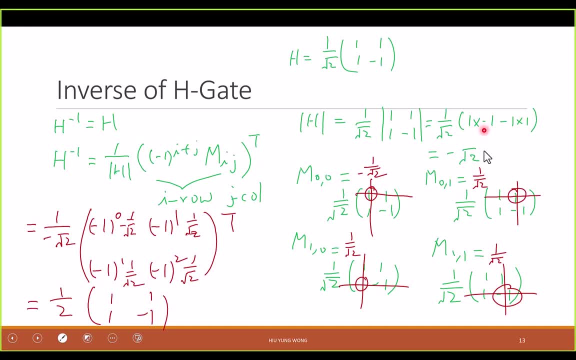 or something 1 times negative, 1 minus 1 times 1. Negative: 2. Yeah Yeah, Yeah, Yeah Yeah. I did something wrong, Very wrong here. The determinant is not this way. It should not be calculated. 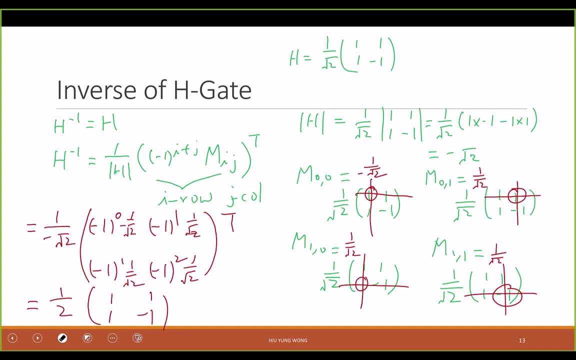 in this way, Because this 1 over square root 2 should go in. Okay. So I did something very wrong. I cannot take out this 1 over square root 2.. Okay, I need to put inside. So that's what happened. 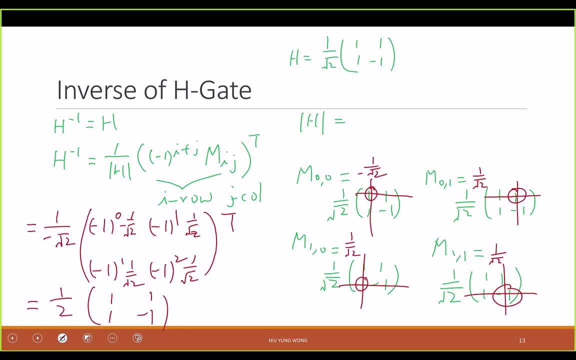 So I should put this as 1 over square root 2, 1 over square root 2, because this is the matrix Correct. So this becomes 1 over square root 2 times 1 over square root 2, which is minus and minus. 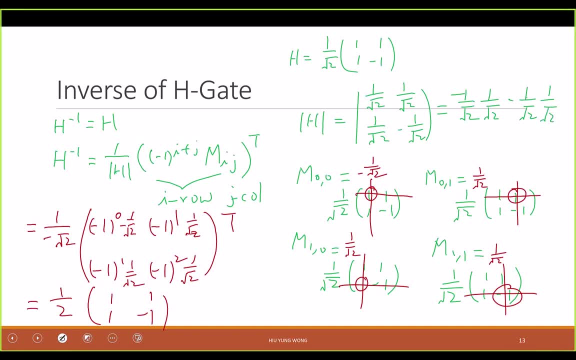 1 over square root, 2 times 1 over square root, 2.. Right, I was using 1 over square root, 2.. So this one gives me what? Uh minus 1.. Thank you, Right, So this is 1. 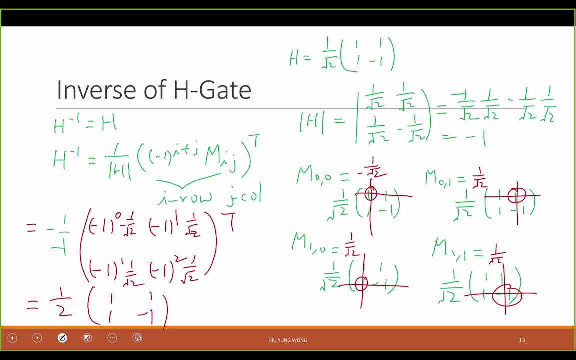 1 over minus 1, And this is if I take out the stuff, it's 1 over square root 2. Right, So this is H? Right? Sorry for wasting your time, but maybe you forget this I don't expect you to do. 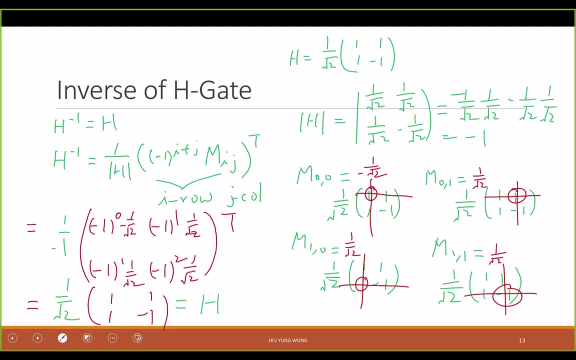 this in the exam. You don't need to know this because it's easy to forget. You can google when you need it, But I really hope you to learn all this problem. Do not like what I'm doing here, Right, Not so straightforward to me to factorize. 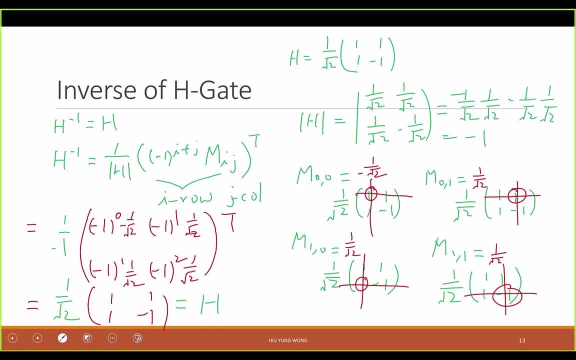 1 over square root L, But it is not So. in the future, when you do this type of program of calculation, be more careful. Don't make the mistake that I'm doing So. my cheat sheet was wrong, But 2 wrongs make 1 right, So my. 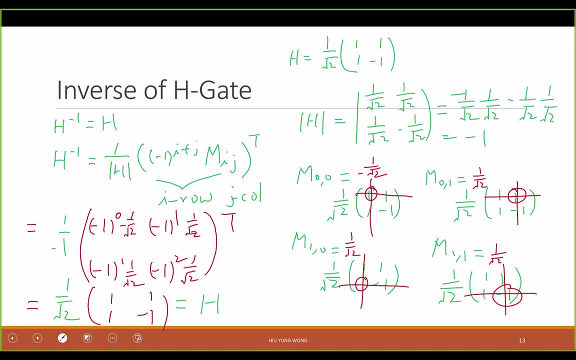 result was correct. That was wrong here and wrong here, But now everything is correct. Yes, Actually, I only grade based on answer. I only check the step if the answer is wrong. Okay, This is a hint. Okay, Very good. 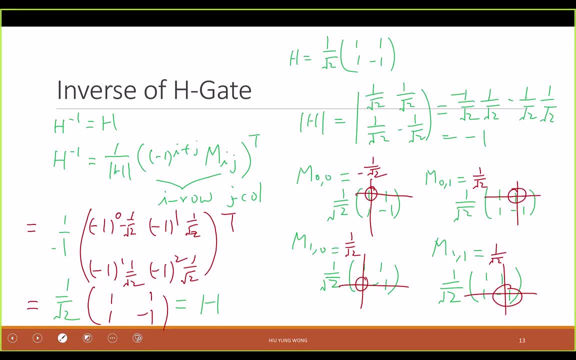 I think we learned something: Just be careful. We learned that we need to be very careful when we play with the matrix. Alright, Good So, but I don't require you to do anything, But hope you train this skill Because in the future, 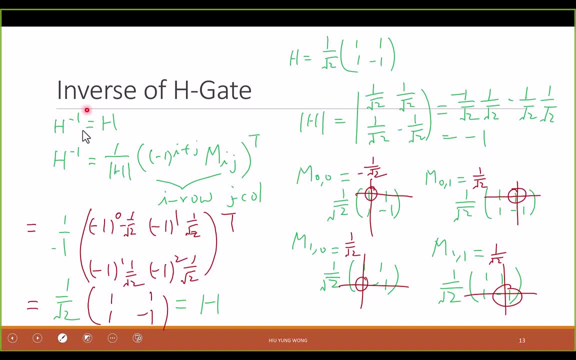 you do linear algebra forever. You need to be careful, Right, But the main point, The only thing you need to memorize for this class, is the inverse of the Hadamard gate equals to itself. Okay, Very important. Now we want to. 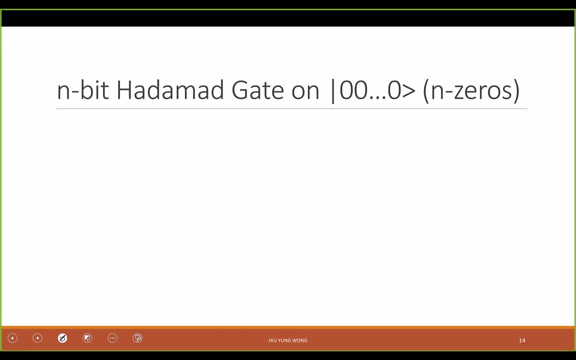 look at some very terrible math But very important. When I apply a Hadamard gate to n qubits, what happen? I already know that when I apply the Hadamard gate to to 1 qubit, it become a superposition Right. 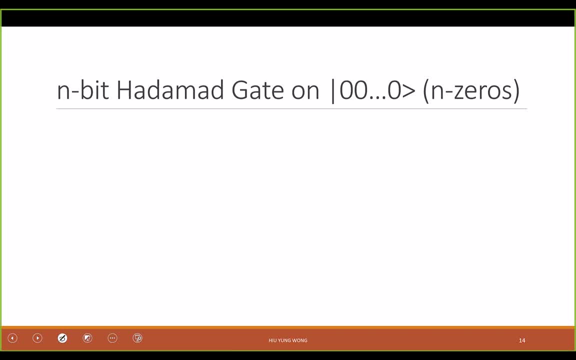 What if it is n qubits? What does it mean? In n qubits of 0 it means right, In a n qubits we have Hadamard gate. I am going to write in this way: Tensor plot the n times. It means n h. 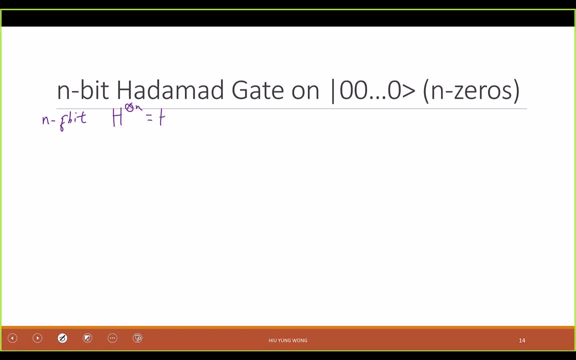 not n tensor product, Right. It means I have h tensor product, h tensor product h, tensor product h and I have n? h Okay, I have n h, Okay. And then, of course, some people write it in this way: That is also okay. 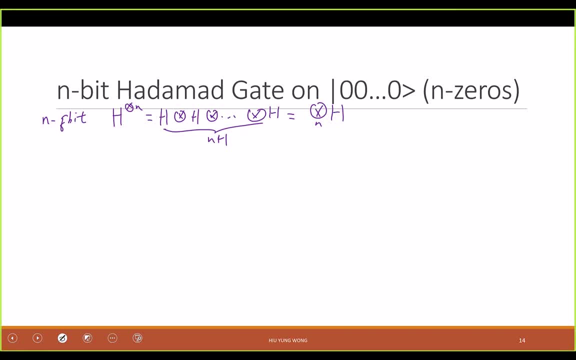 It means n, h, not n tensor product. Okay, You only have n minus 1 tensor product, Right. And this is: what kind of space is this? I have n. what is the space to the power? n d space, Right? Or is the c to the power? 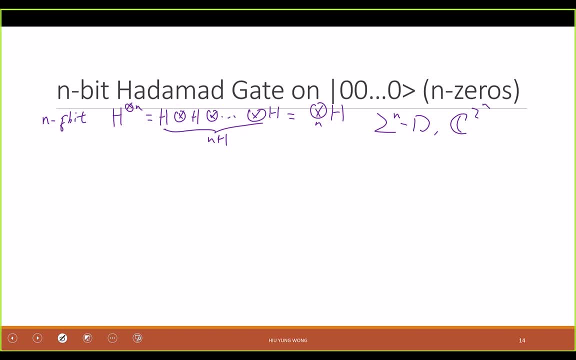 n space. Okay, So I have a function. I want to know what it is when I apply the Hadamard gate to the 0 stage Of this high dimensional space. That is the question here. Can you guess what would it be actually? 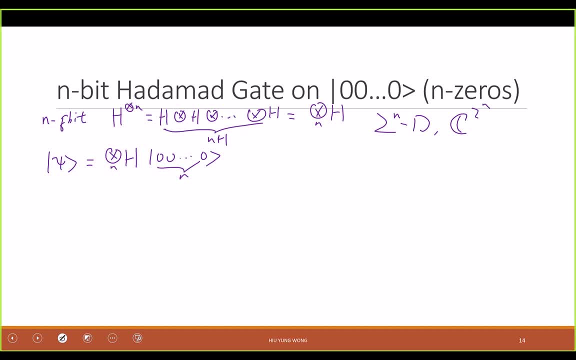 If we apply to 0, it becomes 0 plus 1.. Now I apply to n? 0.. What would it be? A hint is about superposition. Superposition of what? 0 to n. 0 to 0,, 1,, 2,, 3,, 4.. All the. 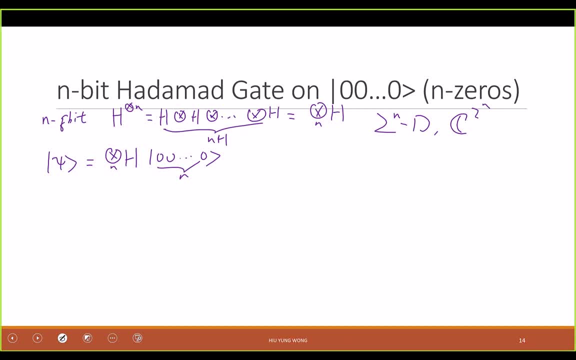 basis states. Okay, In one dimension we apply to 0, it forms a superposition of all basis states. In a: 2 to the power n dimension, right n qubits, it applies to all the basis states That I am going to show you, Right. 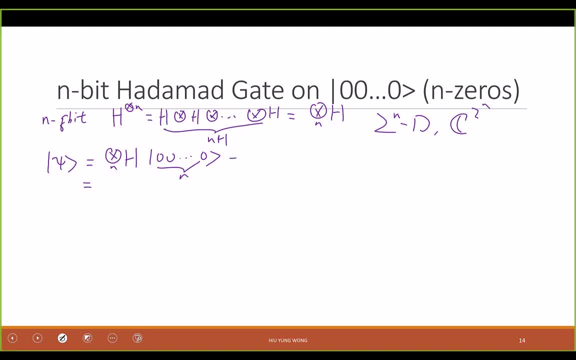 So what is this? Again, we know very well this one is nothing but what. I just write it out Clearly: the so-called n 0 is the tensor product of n 0.. And that's why, for each of the operator, 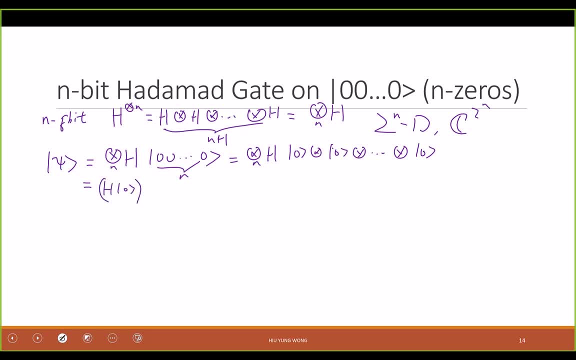 you must only apply to the corresponding space right: The first electron, the second electron, the third electron, all the way to the nth electron Right. Is that okay? We are talking about Huber space. before right, You apply the operator. 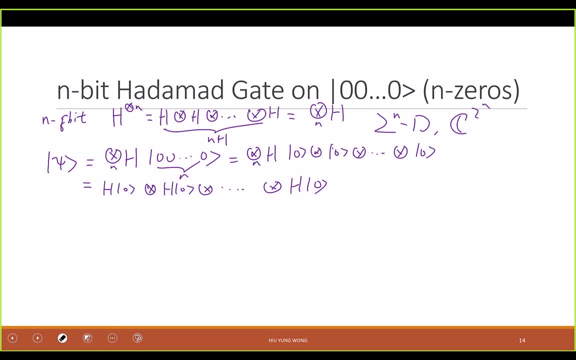 to individual subspace and then you do tensor product. It's the same as you do the vector, tensor product first and then apply the overall operator to that composed vector right. That is what I am doing here. But now I know very. 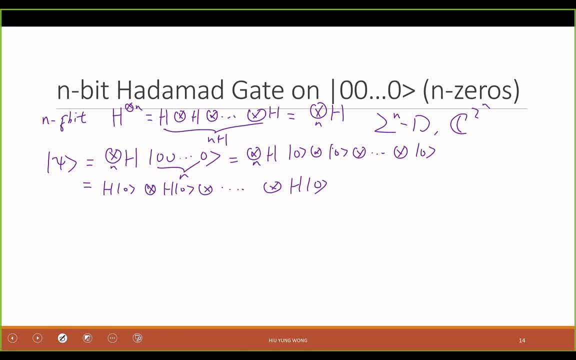 well, what is n? h? n right, What is that Remember? Anyone remember just now? Yeah, yeah, but I apply the h to 0.. What will it be? Becomes a linear combination. yes, Right, This is the first qubit. 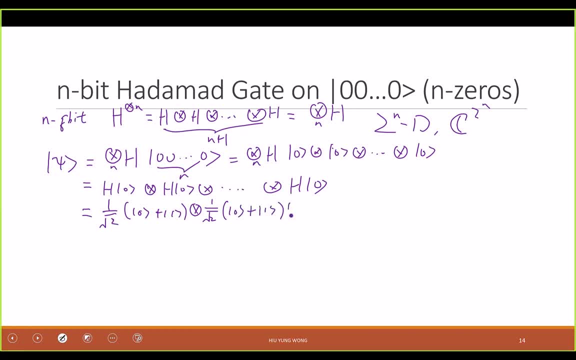 And this is the second qubit, And you will do the same thing for all qubits. All the n qubits Make sense. And then what do you do? Just do a tensor product across them. You obey the distribution law, right? How many? 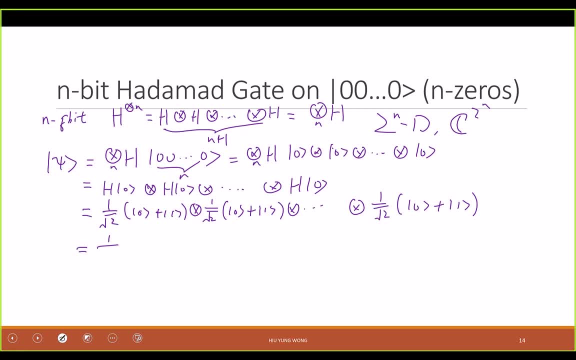 1 over square root 2. do we have, Huh, N only, N only. So it says I can write as 1 over 2 to the power what N over 2. Because it's square root right, So it's divided by 2.. 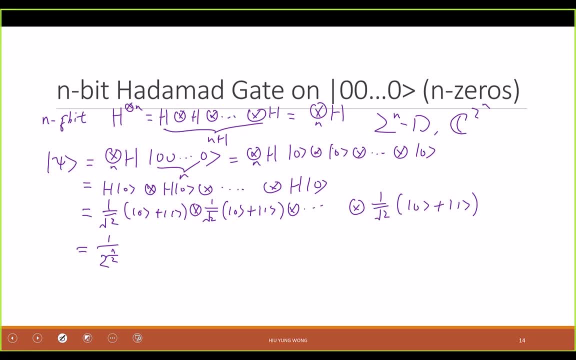 1 over 2 to the power n over 2.. Now let's look at what are the possible combinations I can have: 0 times 0, times 0, all the way, times 0, right, I will just write it out. 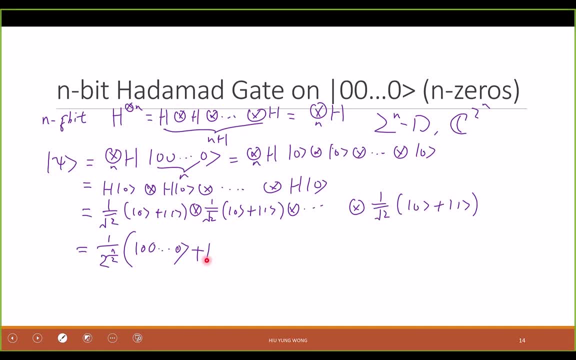 Right, I also can have 0 times 0 times 0, and then the last one I times 1.. And similarly, I can have 0, 0, 1, 0.. And basically, you see that it's just a permutation of all of them And the last. 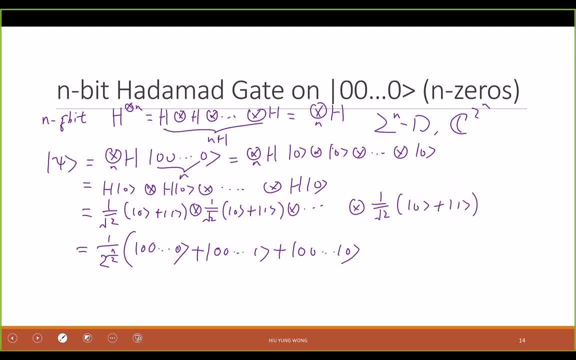 one will be 1 times 1 times 1 times 1.. Before that, it's 1 times 1 times 1 times 0.. Okay, This is in binary representation In decimal. what is this? What is 0??